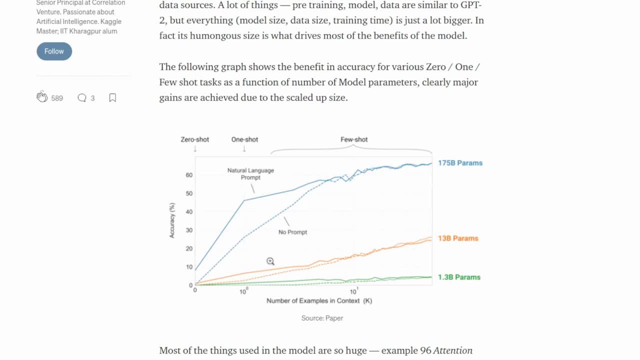 So that is very good. So that is very good. And as we can see with a 13 billion parameter model. It does much better than zero-shot, still not as good as the 175 billion parameter model. 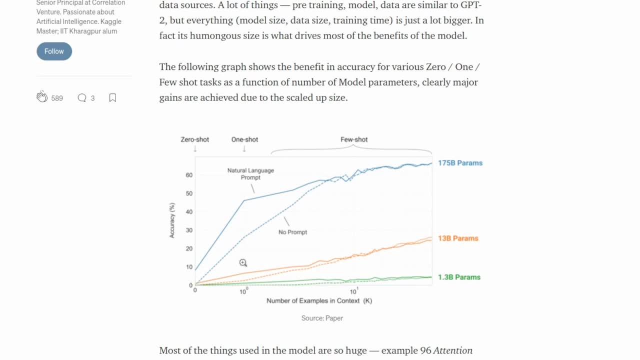 And as we can see with a 13 billion parameter model. You know I did not appreciate that the mouse is not a haha case now. Again, a similar story with the 1.3 billion parameter model. You may be asking though why should I care about this? Well the take-away should be, larger model, tent you do better than smaller models��whis greater model than smaller models. smaller models equally as important is that larger models tend to perform better than smaller models given a limited amount of data thus if we want to fine-tune a model to complete a specific task 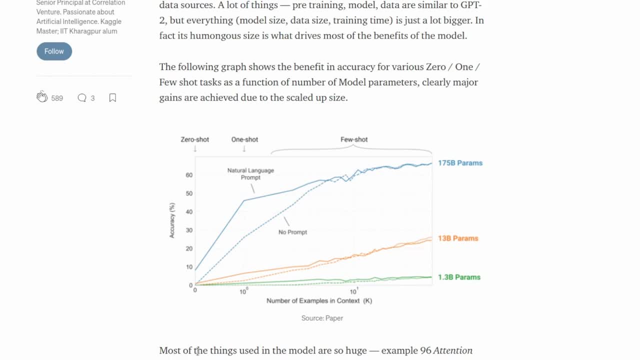 in general we'll be better off using the larger model or the smaller model by doing so we can have a smaller data set to fine-tune on or given a large data set already we'll obtain better results as we can see here so that's exactly what we're going over today how to fine-tune gpt neo 2.7 billion parameters in order to obtain good results on fine-tune tasks like in 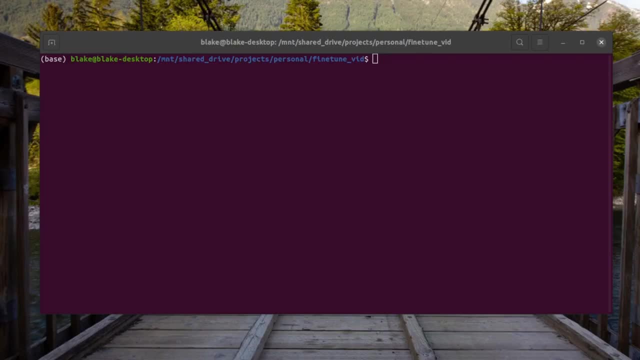 my previous videos we'll be using a jupyter notebook to run the models we will not be using google collab due to the fact that the resources needed to fine-tune these models are too great 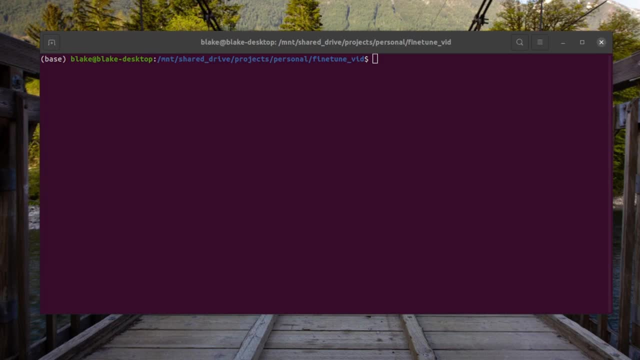 you will want to run this jupyter notebook on your own high-end pc or run this jupyter notebook on a google cloud or azure vm instance with the proper rented hardware to get started then 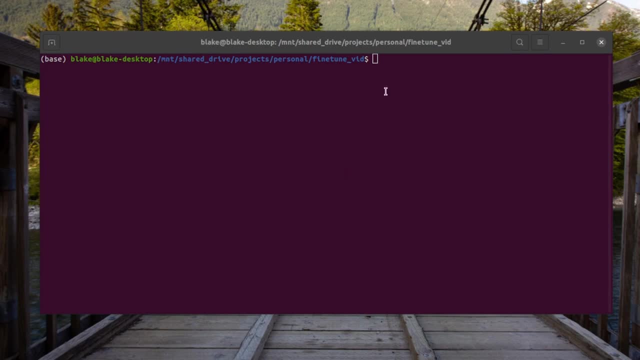 we are first going to need to create a conda environment let's call it conda create in gpt neo fine fine tuned and we'll do python equals 3.7 hit yes 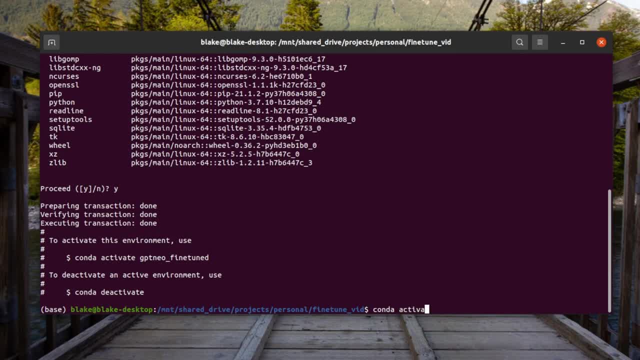 let's now enter that environment so conda activates gpt neofine tuned 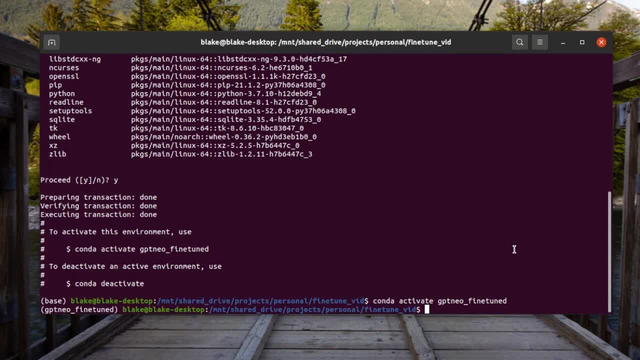 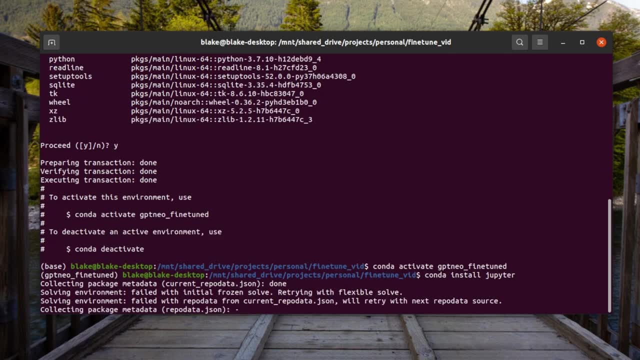 now we're going to need to install jupyter notebooks so we'll do conda install jupyter hit yes 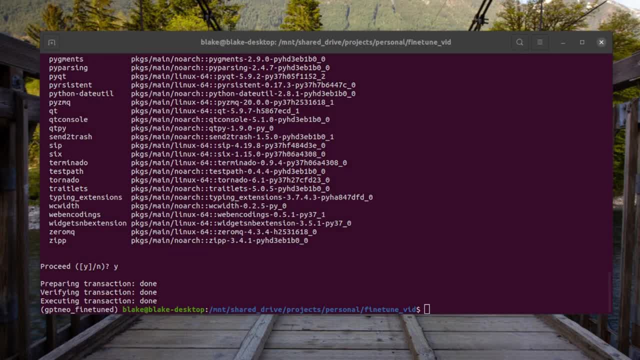 lastly before we go ahead and read it out we enter the Jupyter notebook we need to install a kernel so that our conda environment is accessible inside of the notebook to do this we'll type the following just copy and paste what I have typed here with the main thing 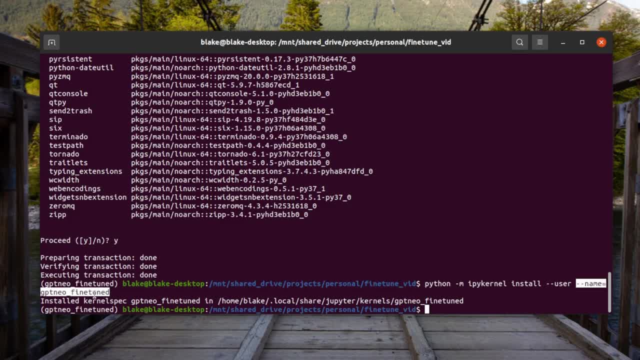 being right here is the name of the kernel and you're going to look for that inside of the notebook before we run Jupyter notebook to launch the Jupyter 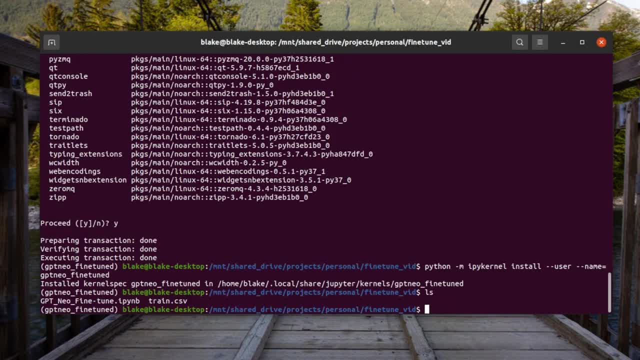 instance let's take a look at our folder we run LS we see the notebook and we also see train.csv this is training data that will be used later so now 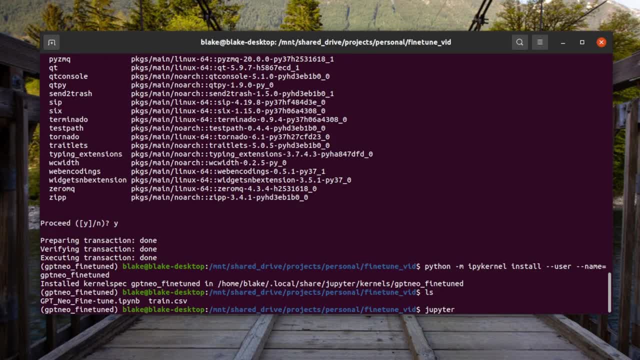 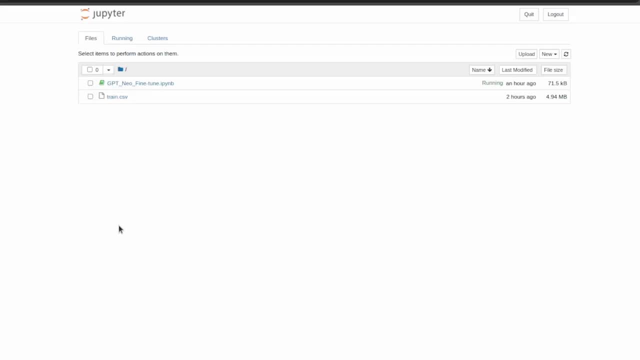 let's run Jupyter notebook and we have started a Jupyter notebook let's go ahead and enter the Jupyter notebook that I have prepared for this video and 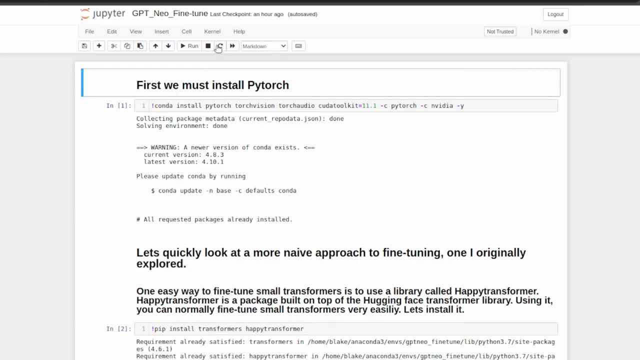 now the first thing that we need to do is we need to run the Jupyter notebook and we need to run the Jupyter notebook and we need to select a kernel so we'll get a kernel change kernel and then we'll 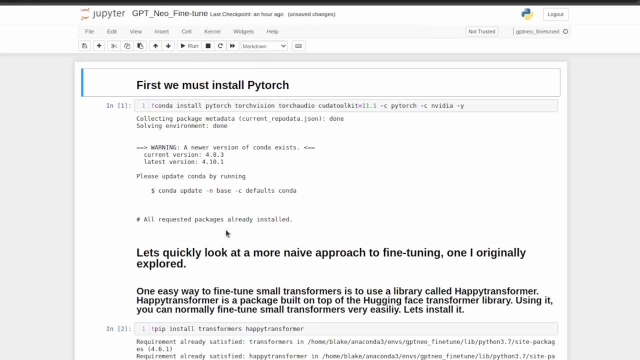 select GPT Neo fine-tuned you may need to now restart the notebook if you're having issues installing packages this may be the fix you can do that by going 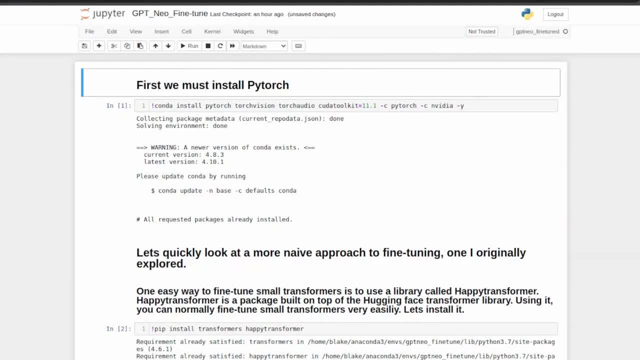 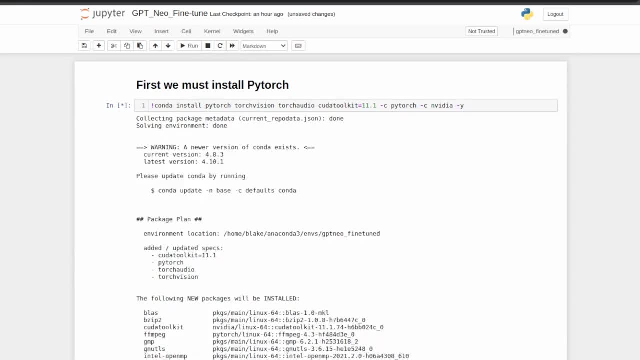 here and hitting a restart so now let's get started with the actual notebook of course we must first install PyTorch so let's go ahead and do that once that's finished let's go ahead and very briefly go 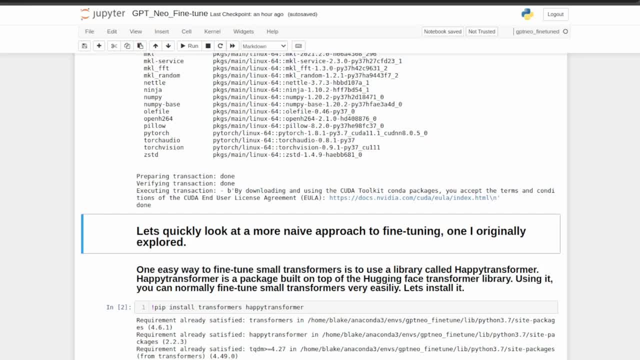 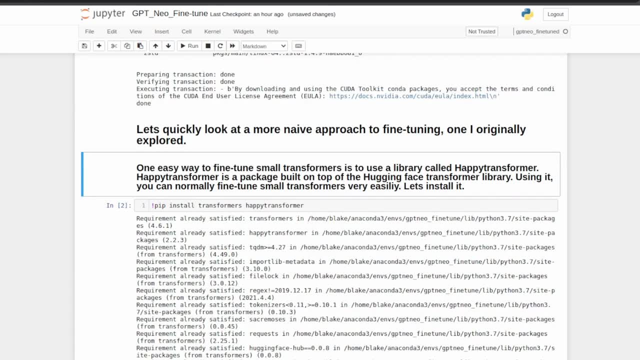 over a more naive approach to fine-tuning these models an approach that I originally explored and had some issues with so one easy way to fine-tune small transformers is to use a library called happy transformer happy 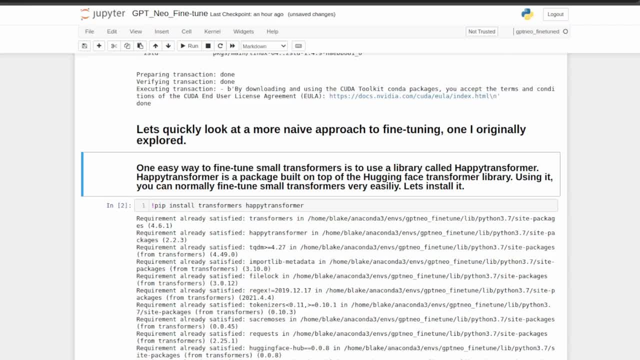 transformer is a package bailed on top of the hugging face transformer library using it you can normally fine-tune small transformers very easily let's install it and see how that works the our use case here 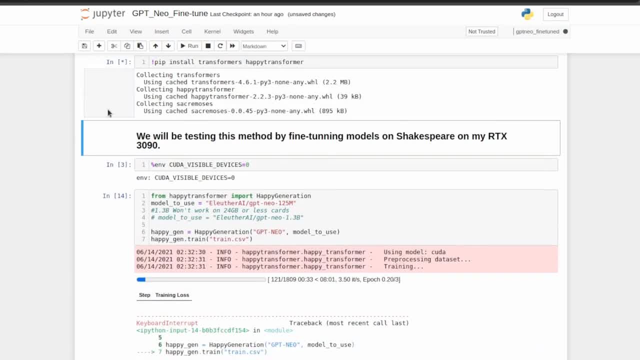 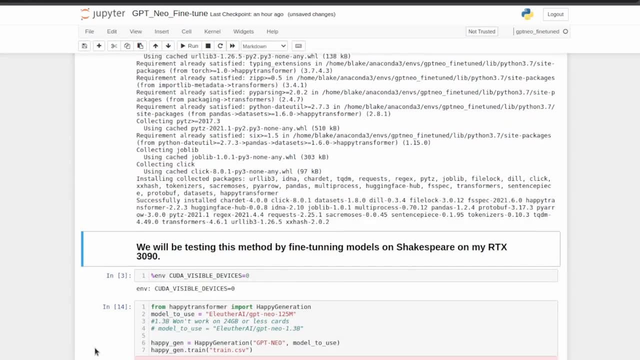 okay now we're installing it and we're done so at this point we'll now begin fine-tuning the models on the Shakespeare data set that I previously 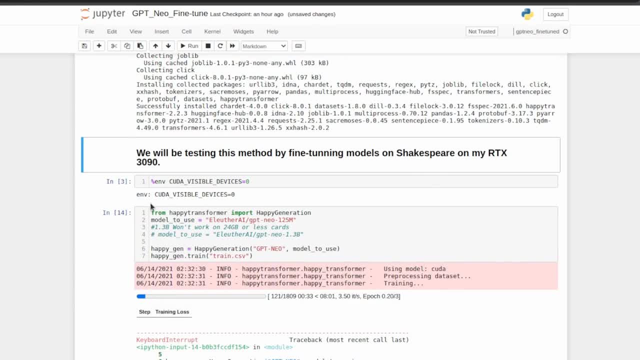 mentioned and we're going to do it on my RTX 3090 that has 24 gigabytes of VRAM so what we're doing now is we're going to set a CUDA visible device to zero so 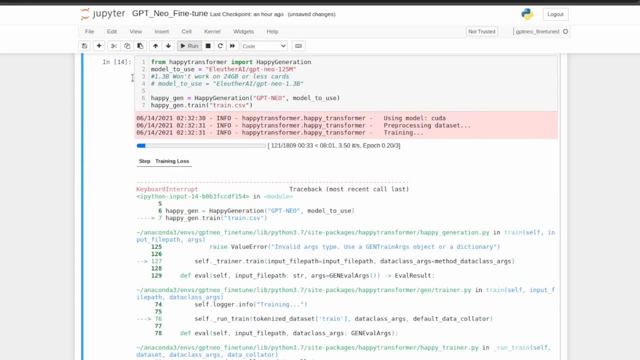 it only runs on my RTX 3090 that's done so what we're going to do here is at first we're going to train on 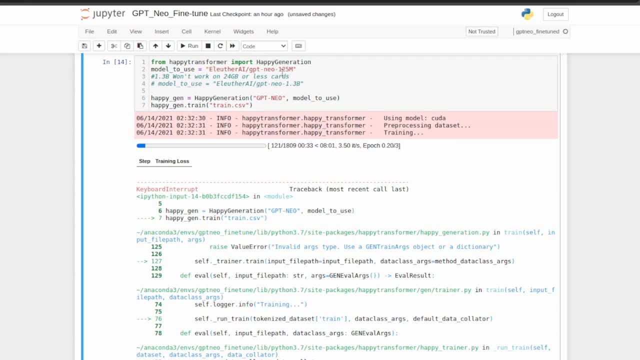 the smallest gbt neo model that is the 125 million parameter model and we're going to fine-tune that model with that trained CSV file containing Shakespeare 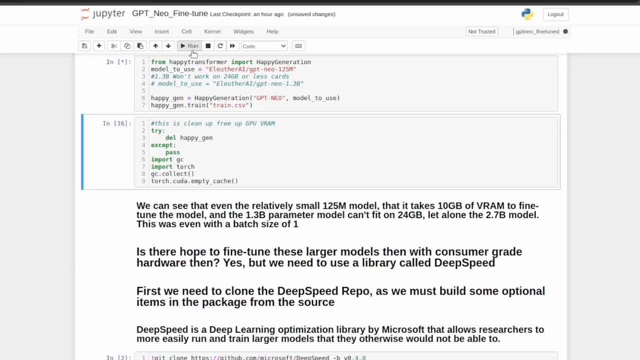 so let's go ahead now and run this segment and it's going to be loading the model here soon 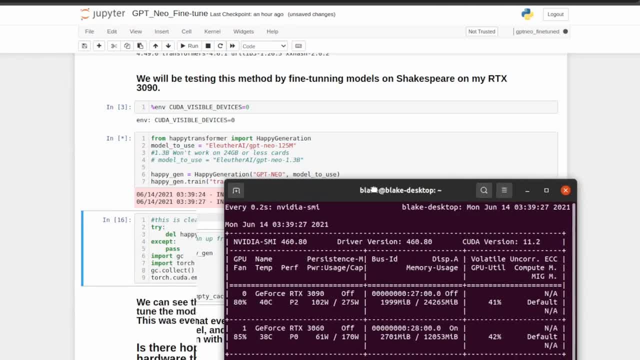 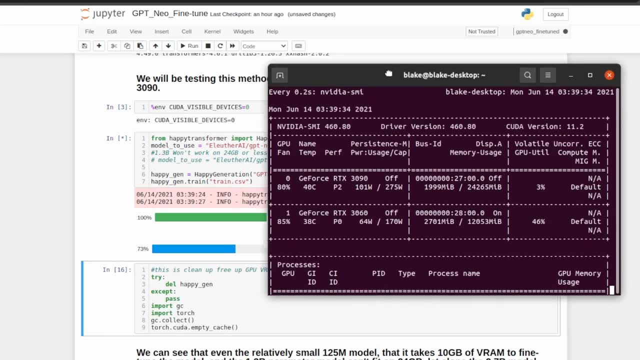 so as we can see right here is we see an NVIDIA SMI and we see the VRAM starting to get filled up so that two gigabytes and now it's training and see we see it 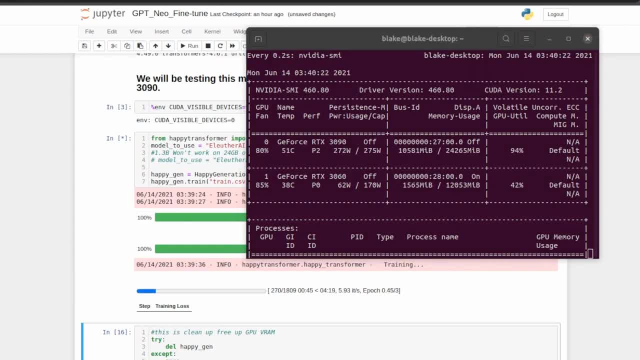 jump to 10 gigabytes here what this means is that in order to train even just the 125 million primer model with the batch size of one we need a GPU with 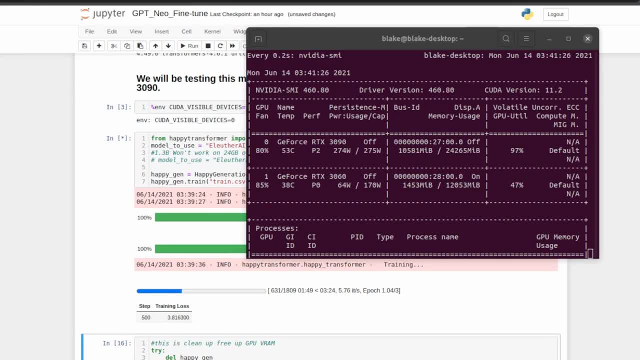 at least 10 and a half gigabytes of ERAM this unfortunately eliminates many cards from being able to be used to train even the 125 million parameter 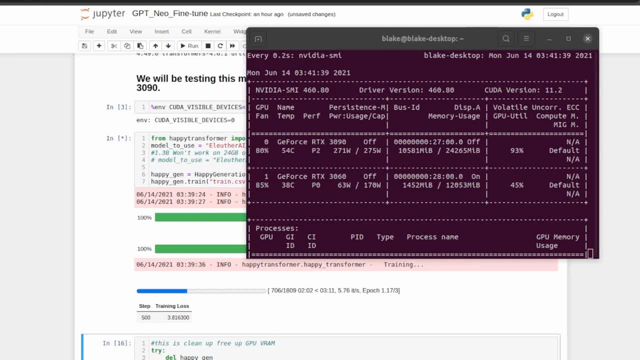 model this will eliminate the RTX 3080 3070 ironically the 3060 would be able to do this the RTX 3080 Ti will be able to do it the GTX 1080 Ti would be able to do it and the 2080 Ti would be able to do it and of course the RTX 3080 Ti will actually race the 256 number or so GTX1080 Ti or the 4840 succeeding on the 11lets. so it looks like this is it for an aesthetic result now let me show you what that is so here at the sweat no display conditions but we're able to страшly it starts to split anyways end disconnect the GPU My vaccination and cancel the calculation could begin an accident 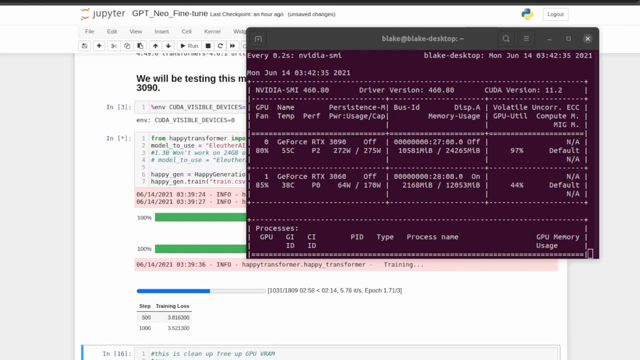 x3090 will be able to fine-tune the model but that is it with regards to consumer cards so at this 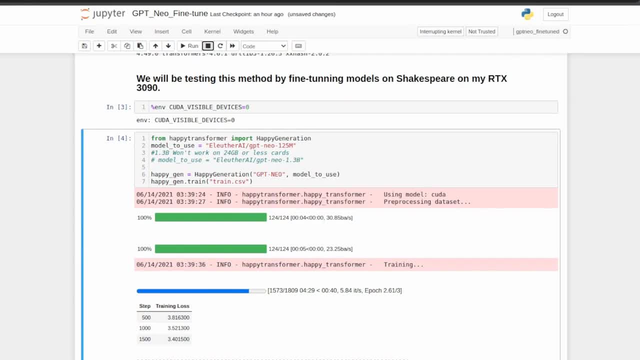 point let's go ahead and stop this early we know how much vram it uses and we don't want to use the 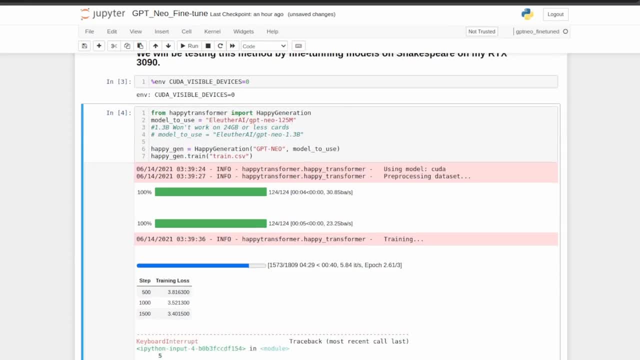 125 million primer model anyways and now what we need to do is we need to run this segment right 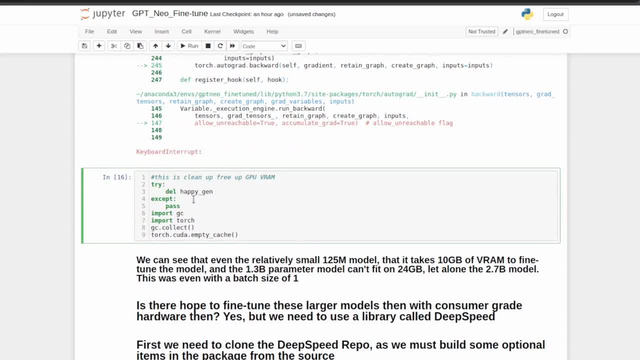 here but this segments going to do is it's going to clear the vram usage for the GPU and will allow 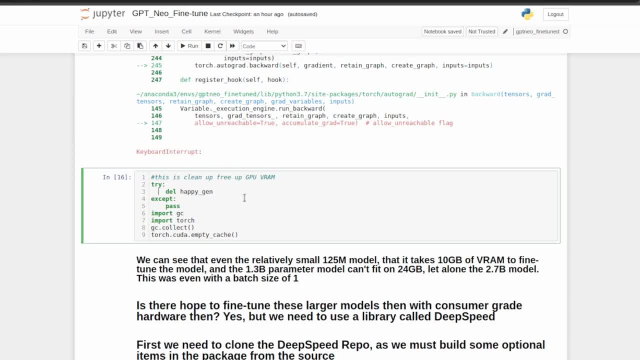 us to again run the above code segment but this time we're going to see how it performs with the 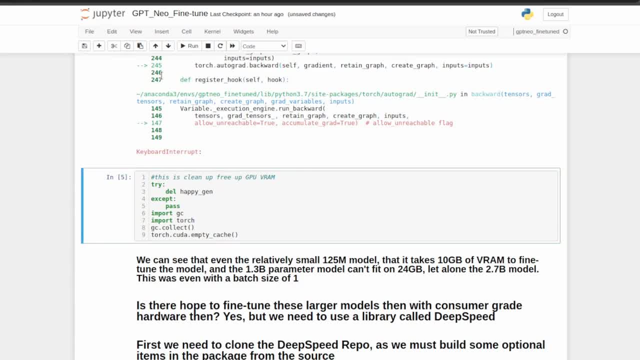 1.3 billion perimeter model so now we're going to run this section here and now our vram should 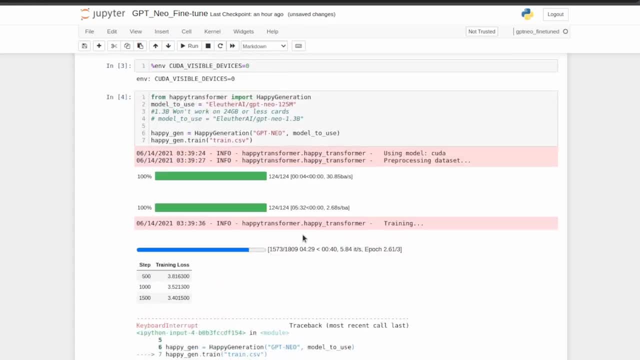 be cleared so now let's go back up to the code block that was training 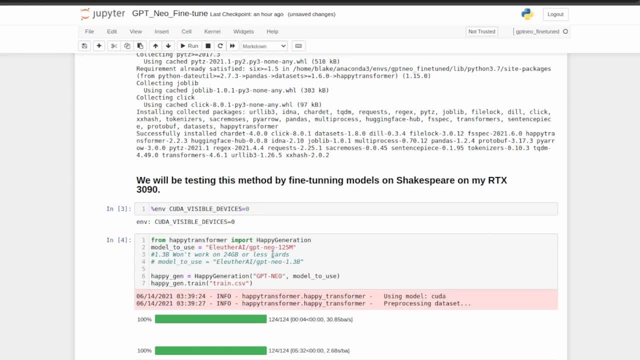 the 125 million primer model and let's change it to 1.3 billion parameters spoiler this is going 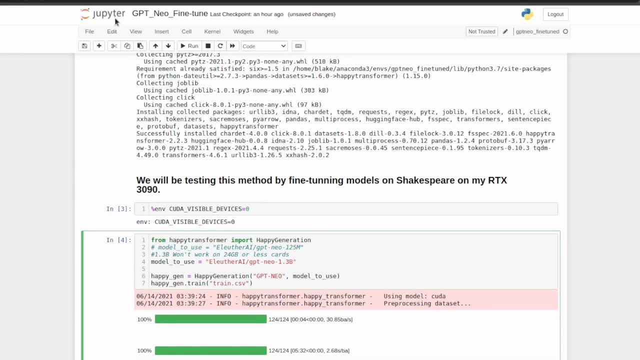 to error out but let's just see what it does exactly so now I'm going to run this here and 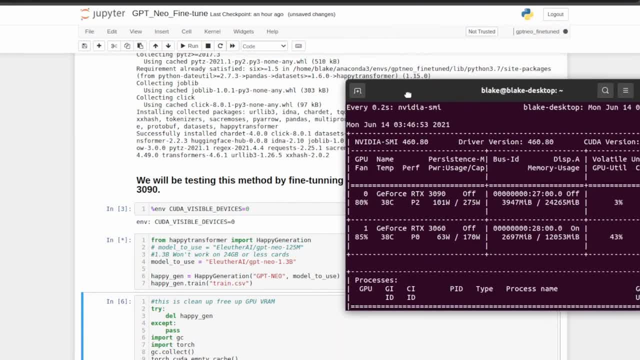 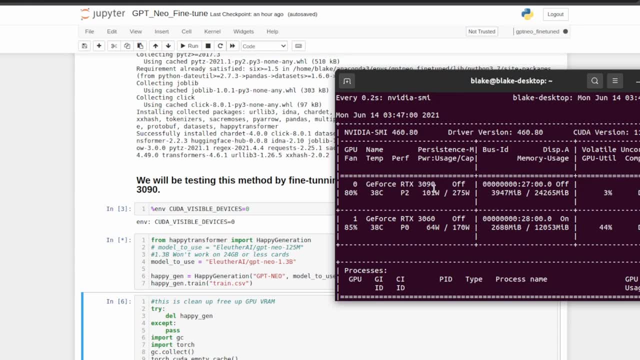 let's keep an eye on the GPU vram usage should be loading here any second now 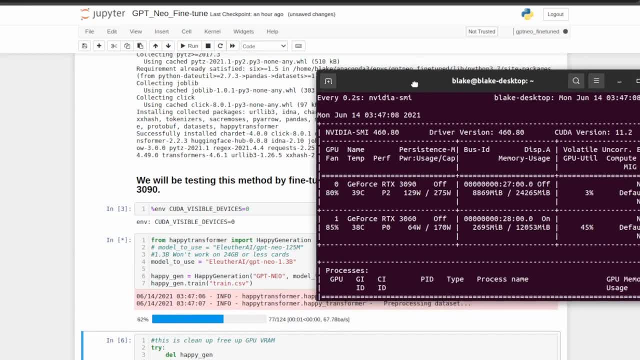 let's go back to the vram and let's see what it does okay it's at 8 so it's 8 before we start running 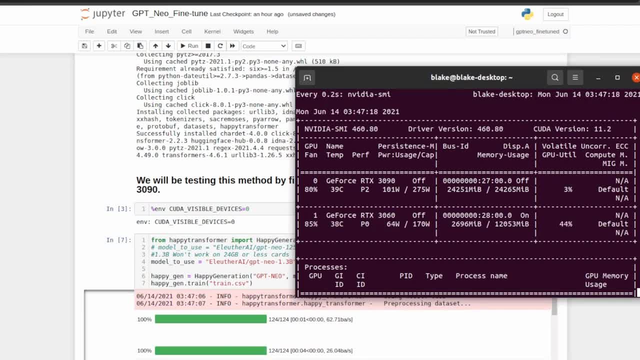 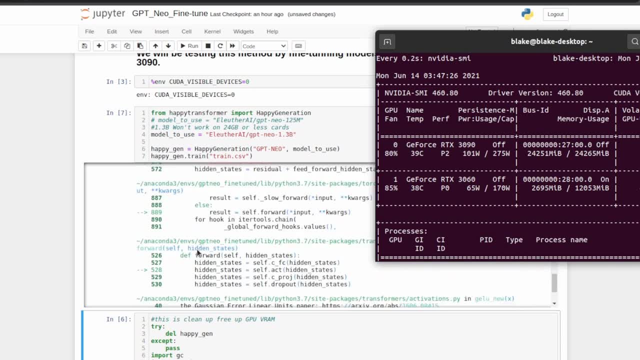 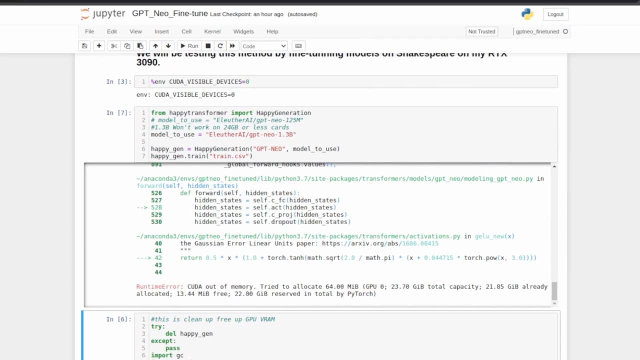 now it's at 24 and maxed out and we will have an out of memory error if we scroll down let's see it right here out of memory so as we can see while happy Transformer makes it very easy to train small Transformers 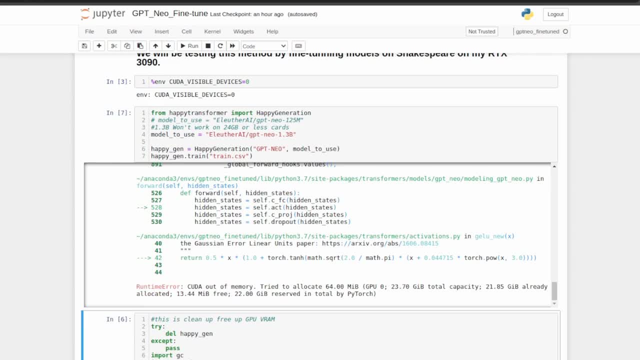 it is insufficient for the 1.3 billion parameter model and even more so for the 2.7 billion parameter model and as I talked in the beginning of the video we want to fine tune on large models 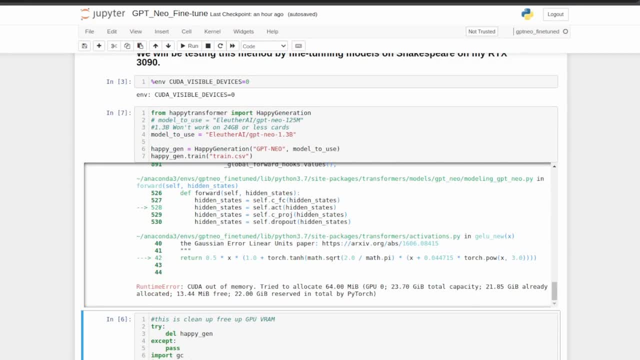 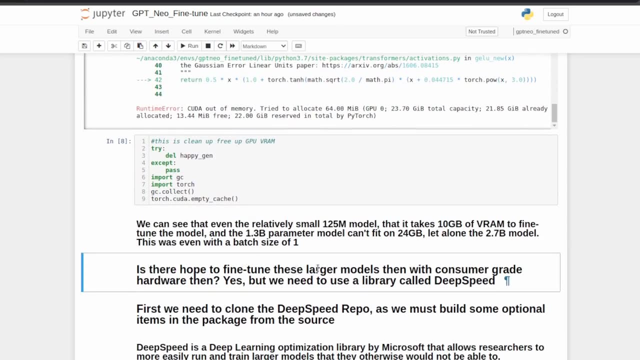 because large models are able to learn better and with less data compared to smaller models so then is there any hope that we can train these larger models with consumer grade hardware fortunately the answer is yes but we need to move 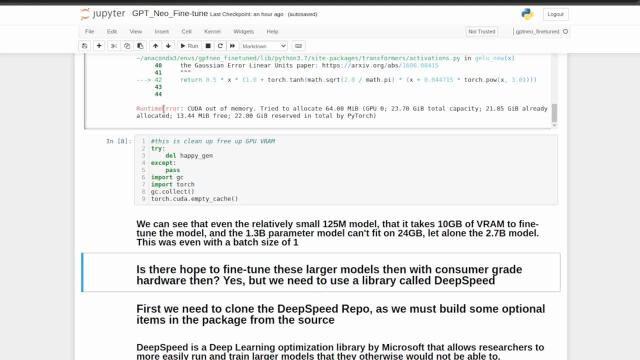 to a different library we need to use deep speed first we need to clone the deep speed repo as we must build some optional items in the package from the source deep speed is a deep learning 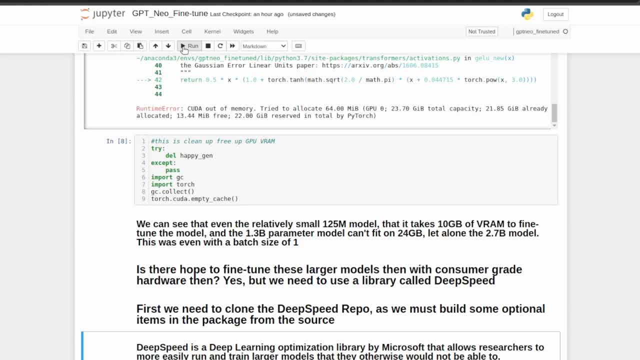 optimization library by Microsoft that allows researchers to more easily run and train larger 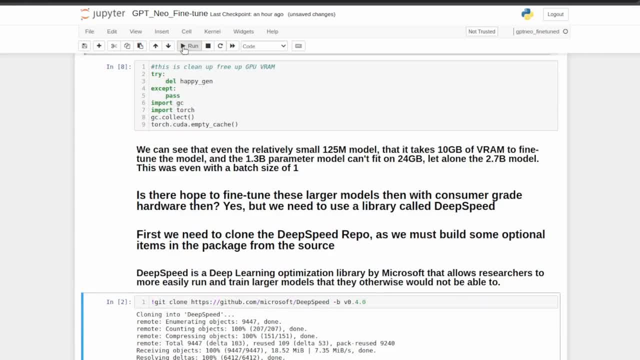 models that they otherwise would not be able to do so by running this block here we'll go ahead and clone the repo 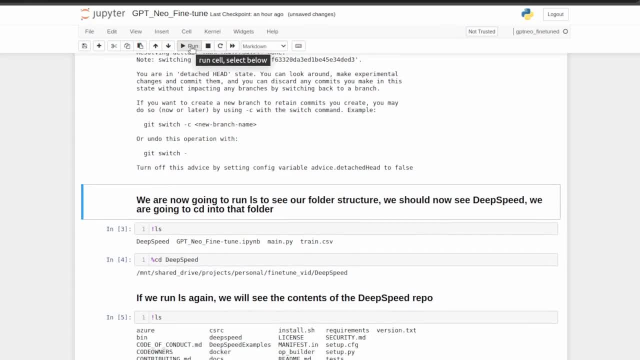 and that's done and so now if we LS our folder structure we see that deep speed is located in 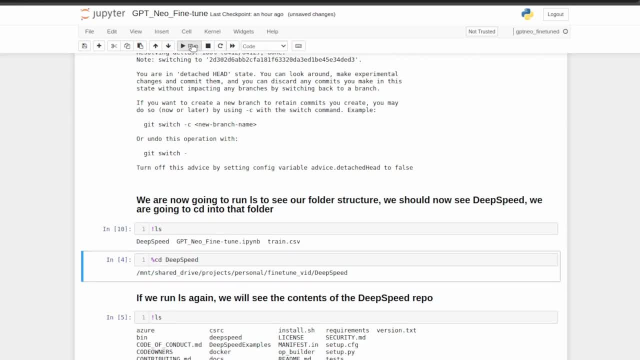 the folder we now want to CD into deep speed and now we've done that again if we LS the folder we 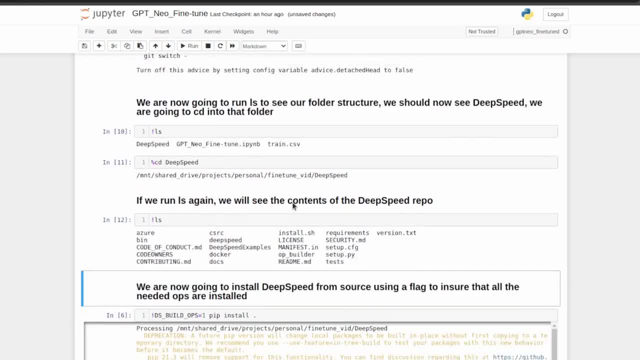 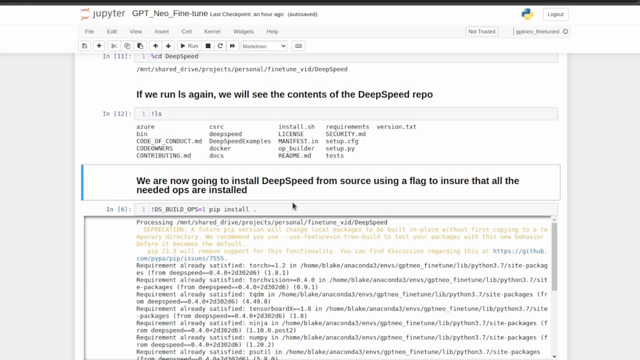 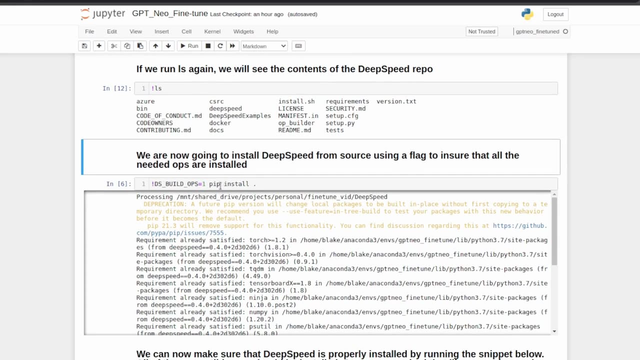 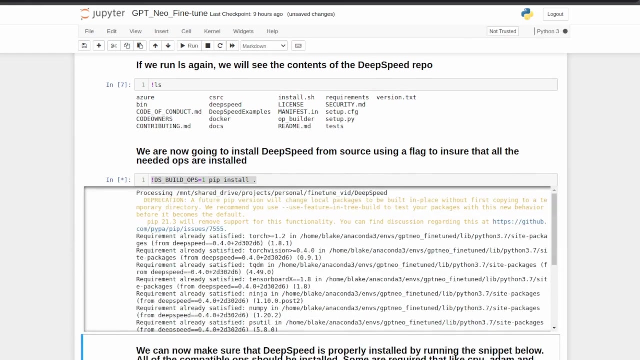 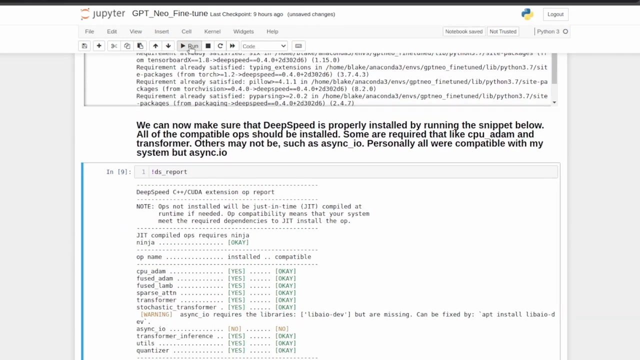 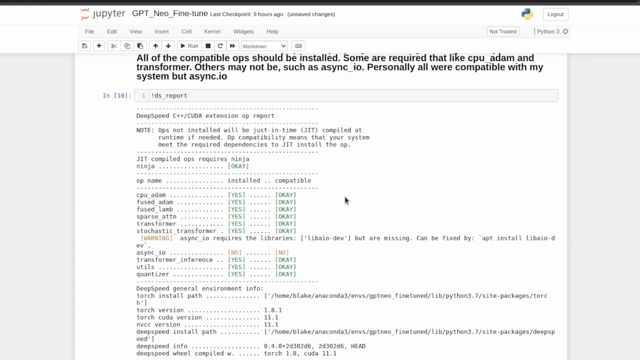 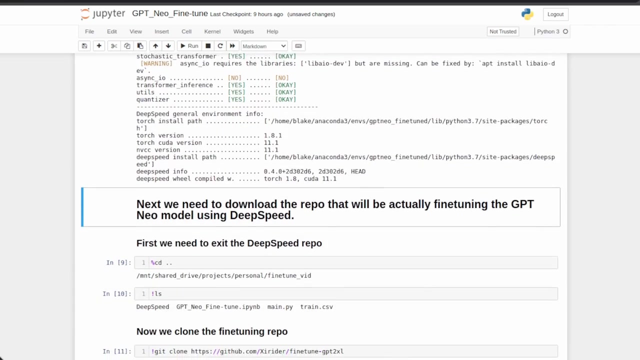 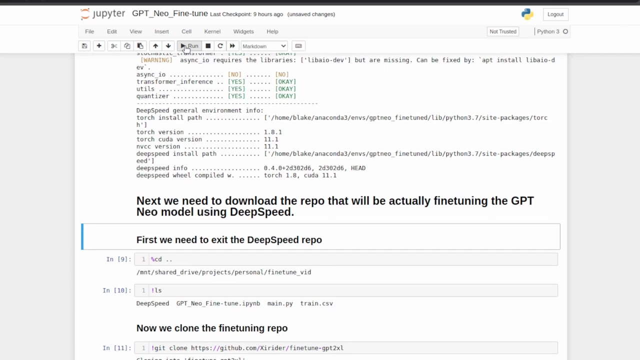 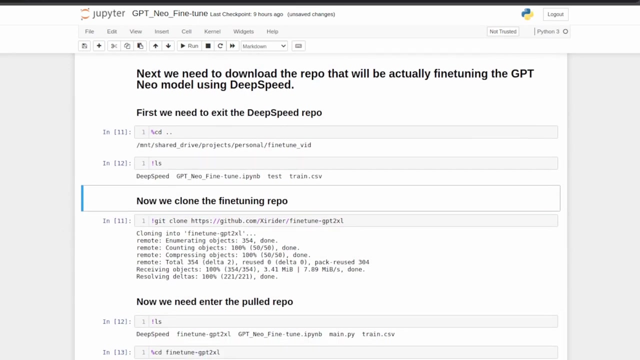 will see the contents of the deep speed repo so now the next step is to install deep speed from source using a flag that's in the documentation to ensure that all needed Ops are installed to do this run this command here ds build ops equals one pip install period period meaning the current directory so let's do that now installing deep speed from source may take a while on my computer it took over six minutes but just wait it out and you should be good to go once we have deep speed installed the next thing we're going to want to do is run ds report so what ds report does is it lets you know if the compatible ops are installed on your pc i'm not quite sure which all ops need to be installed but i can tell you for sure that cpu atom needs to be installed ninja as well as transformer i can tell you that async io does not need to be installed these are the ones that are compatible with my system and with these ones installed i can get deep speed to work after we do that we need to now download the repo that will actually be installed on my computer and i can tell you for sure that cpu atom needs to be installed actually be fine tuning gpt neo using deep speed so let's first exit the deep speed repo repo by doing cd dot dot you can run ls now to see that we're back on the above folder and so what we need to do now is we now need to clone the repo for fine tuning to do this 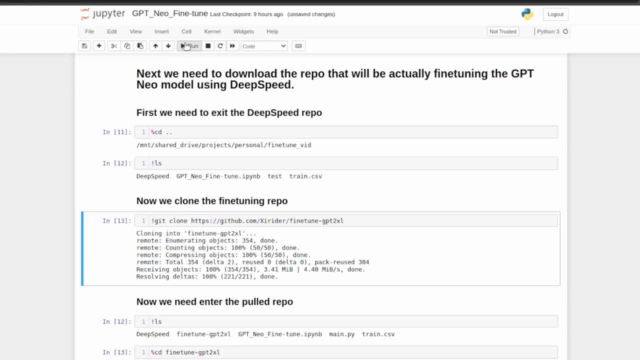 we'll just simply run the code block here to download and clone the fine tune gpt2xl repo and now that it's done we can see that it is 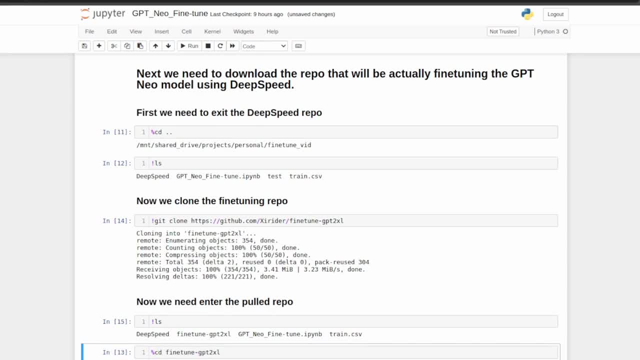 in the main folder so now let's enter it by doing cd fine tune gpt2xl 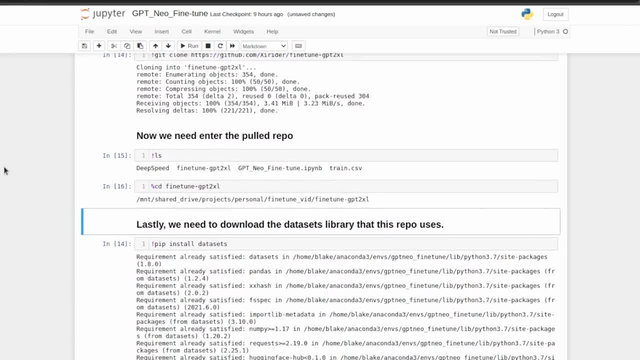 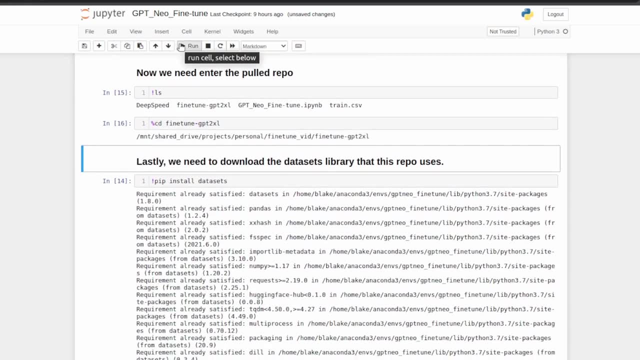 so the last thing that we need to do now that we're inside of the fine tune repo is we need to download and install the data sets which is used in this repo 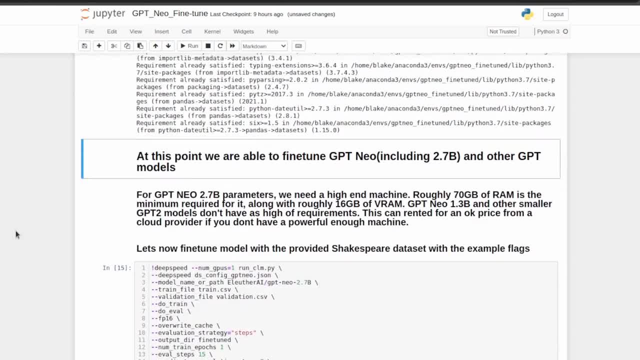 and we'll do that so now at this point we're able to fine tune into the repo and we're able to do that so now at this point we're able to fine tune into the repo 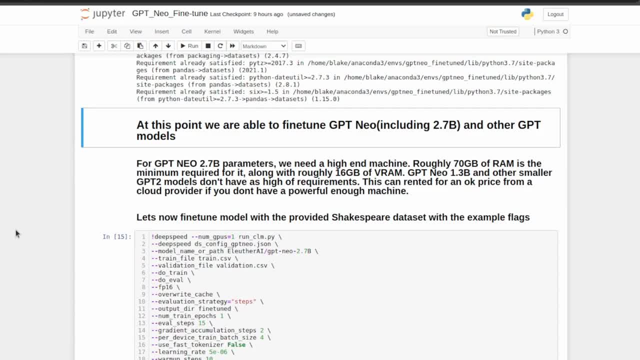 gpt neo including the 2.7 billion parameter model as well as other gpt models such as gpt2 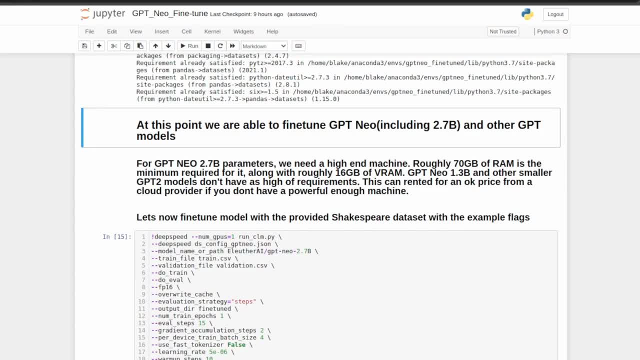 gpt2xl etc so for gpt neo 2.7 billion parameters we need a high-end machine the readme says that 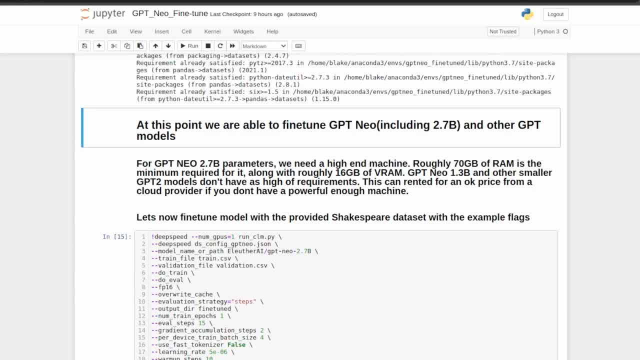 roughly 70 gigabytes of ram is the minimum required for it along with roughly 16 gigabytes 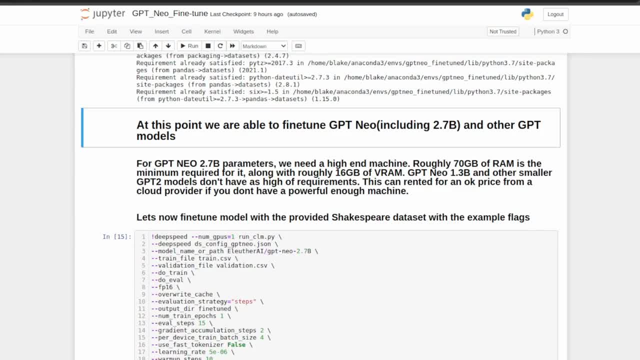 of vram on a gpu gpt neo 1.3 billion and other smaller gpt 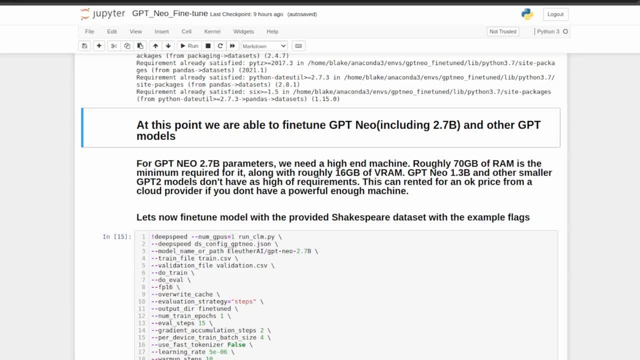 2 based models don't have as high as requirements this can be rented for an 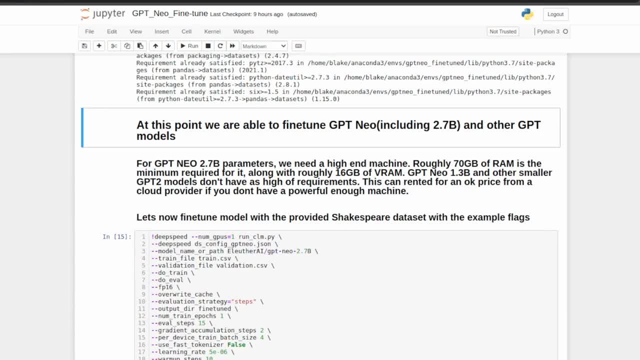 okay price from a cloud provider if you don't have a powerful enough machine normally the cost to rent a machine to do this for a month would be a couple hundred dollars but to fine-tune a model you'll probably only need to rent it for 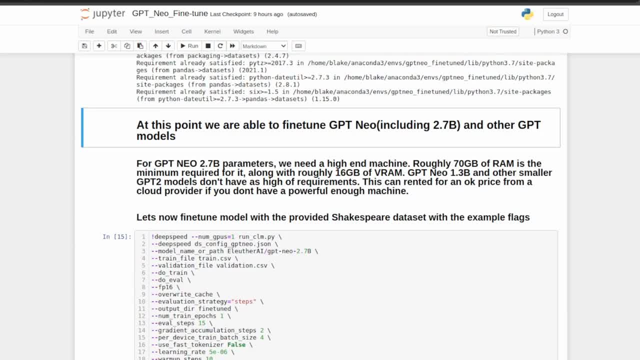 a couple hours so it's probably around ten bucks at most personally I had to upgrade my PC from 64 gigabytes of RAM to 96 gigabytes of RAM just in order to 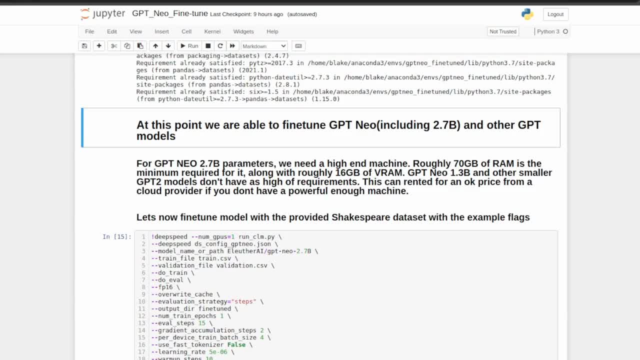 make this video and do some cool things with gpt neo 2.7 billion but as I've gone over in my previous videos once you have a trained model you can run that 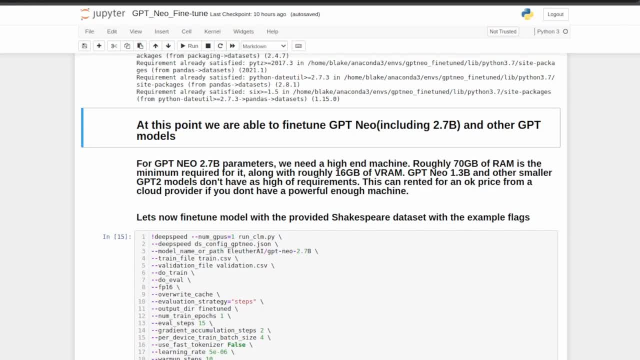 trained model on much lower-end hardware even with just a CPU as long as you have a decent amount of RAM so now let's go ahead and fine-tune gpt neo 2.7 billion 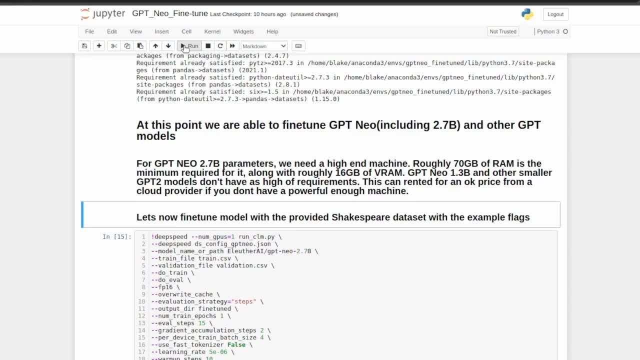 with the Shakespeare data set that I mentioned earlier the flags are gonna be using here are the ones in the readme that I highly recommend you read 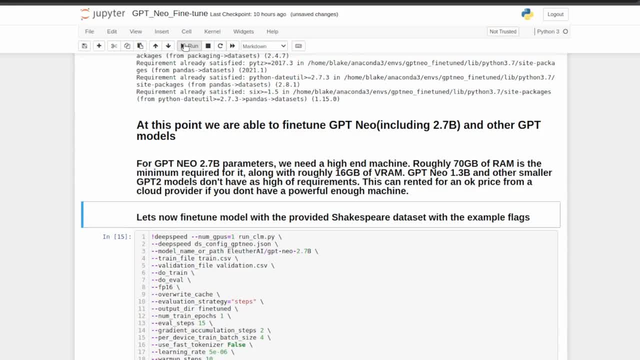 yourself and this will supposedly work on 16 gigabytes of VRAM and roughly 70 gigabytes of RAM I can personally say guarantee that it works on an RTX 3090 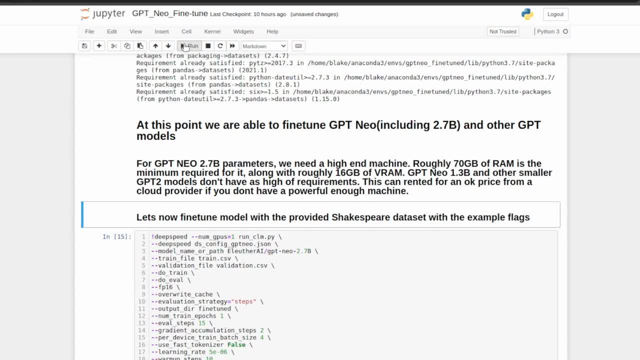 and 96 gigabytes of RAM but as you can see you almost certainly can get away with much less once you run this code block here it'll take a few minutes to get started once it does 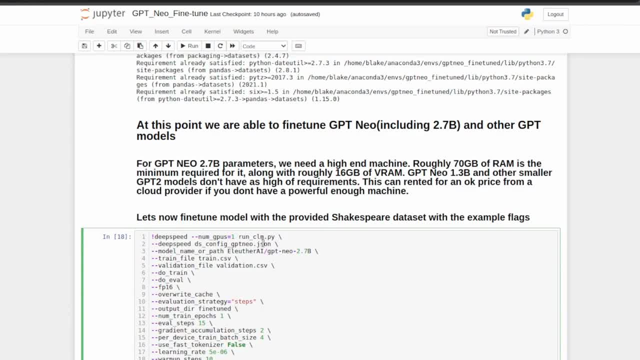 it'll take a couple hours to fine-tune the model depend upon several factors such as number of train epics batch size parameters and flags that you can set on 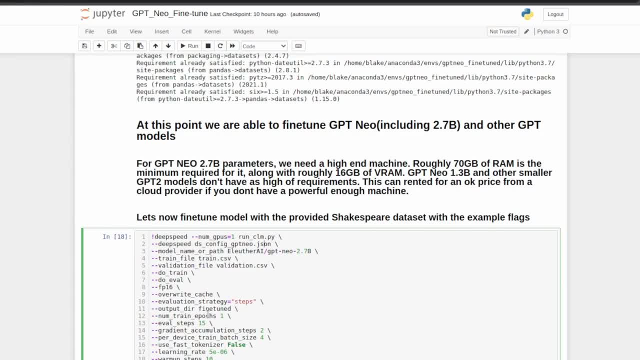 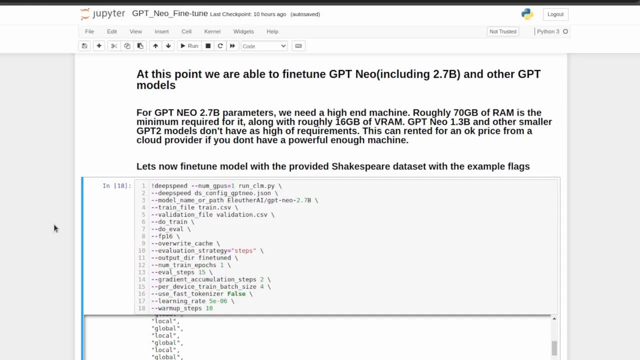 your own depend upon your own hardware and requirements let's go ahead now and run this code block and check out how it's affecting my computer how much RAM 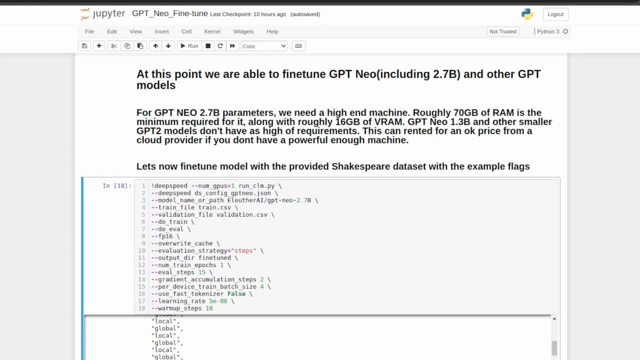 it's using how much VRAM it's using and see what the impact is of running this model so now I've just started the process 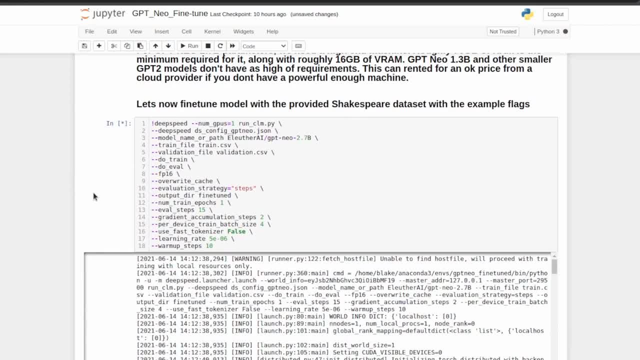 of fine-tuning the model I'm going to now skip ahead until it actually starts training so we can truly see the impact that training the model is having on our 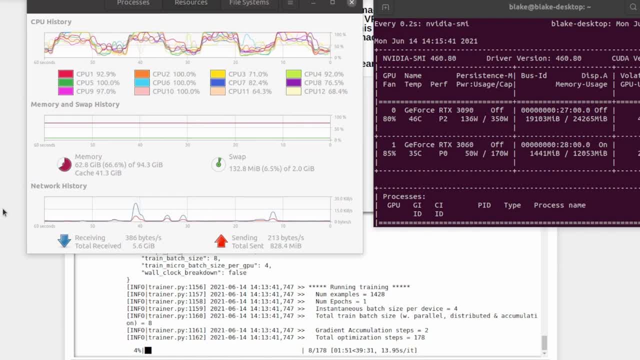 hardware what resources are we using we're now into the process of training 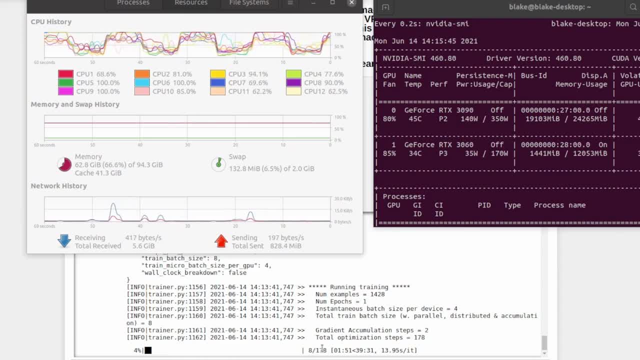 we see we're on step 8 of 178 just the way that the data is batched up with this model we can see that we are using 19 gigabytes of VRAM and 63 gigabytes of RAM 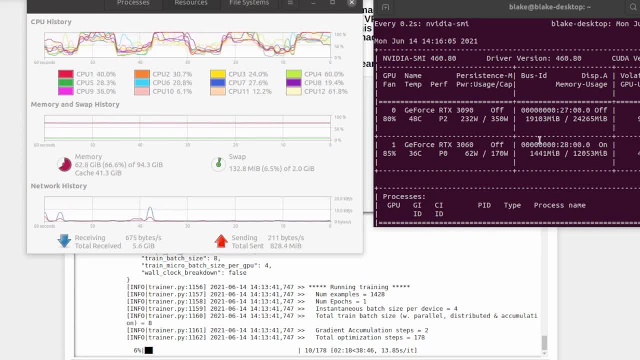 the reason that we're using 19 gigabytes of VRAM is due to the fact that we have 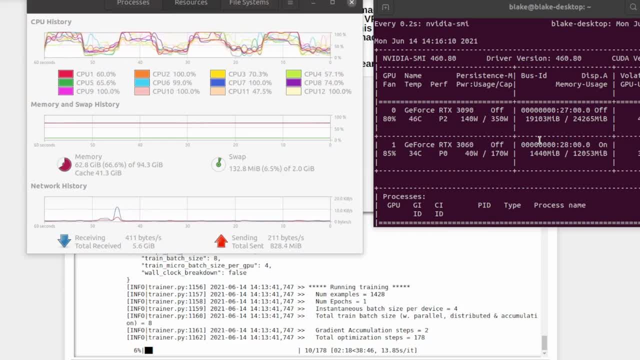 the resources available if we had a less VRAM my understanding is that we would be using more RAM although I could be wrong about that the last thing we're going to 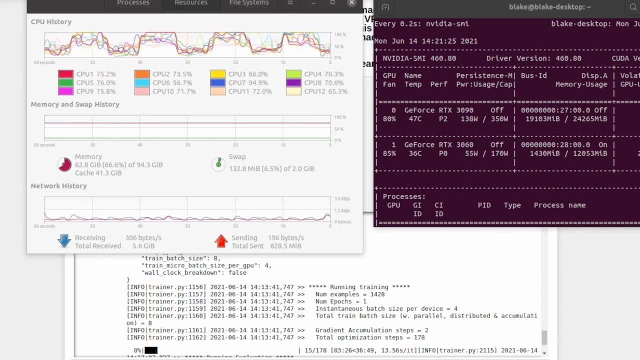 do with this notebook is I'm going to kill the training process and then reload 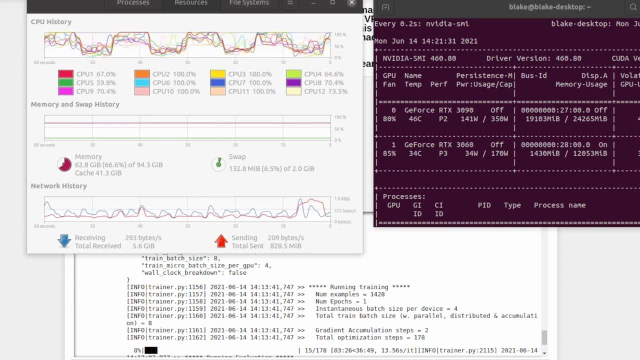 the training process but with different parameters so that we can further reduce the hardware demands I have now restarted the notebook and we can now change some of 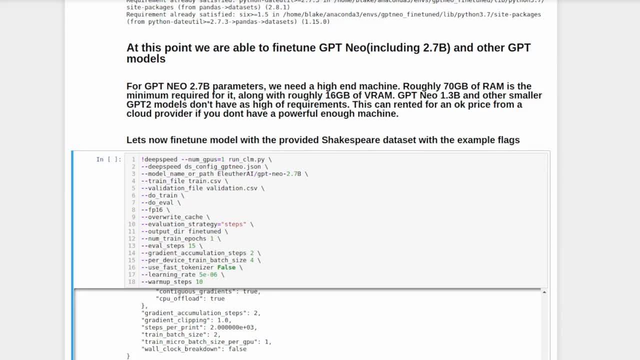 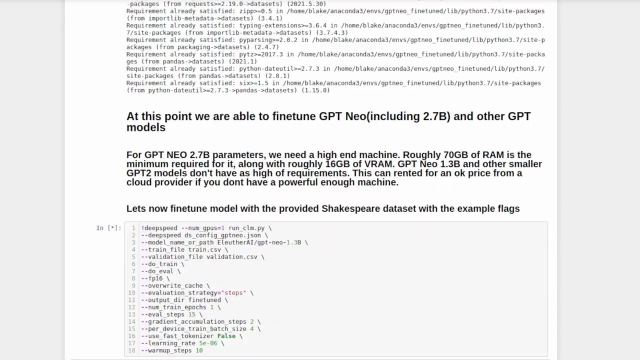 the tags one of the more obvious ones is that we can change the model we use from 2.7 billion you can change that to 1.3 so now let's run that and let's see what kind of performance 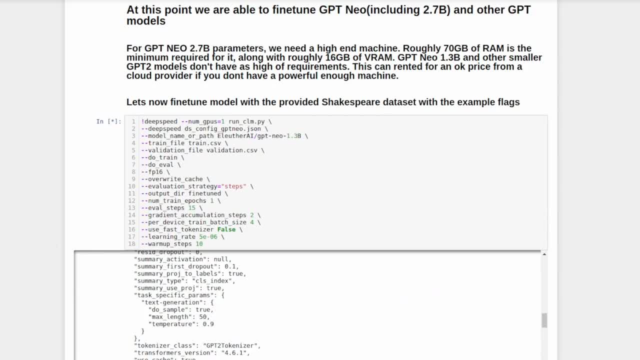 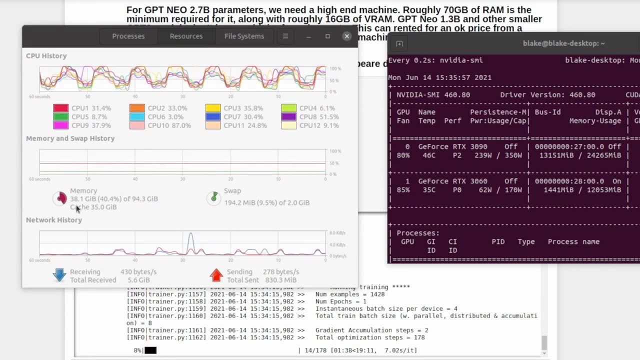 impact on our hardware we see so right here we are training a GPT Neo 1.3 billion parameter model we can see he's using significantly less RAM he's in 38 gigabytes it's also using significantly less VRAM 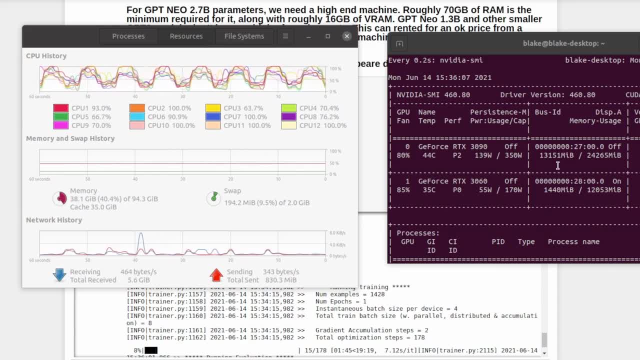 he's using 13 gigabytes so we can see that of course the 1.3 billion parameter model requires less powerful hardware to fine-tune and you can definitely do this on more mid-range hardware or 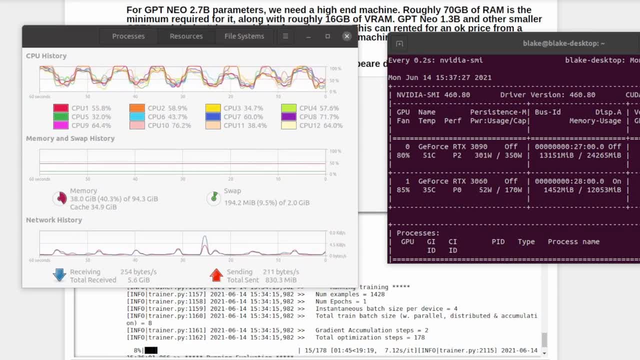 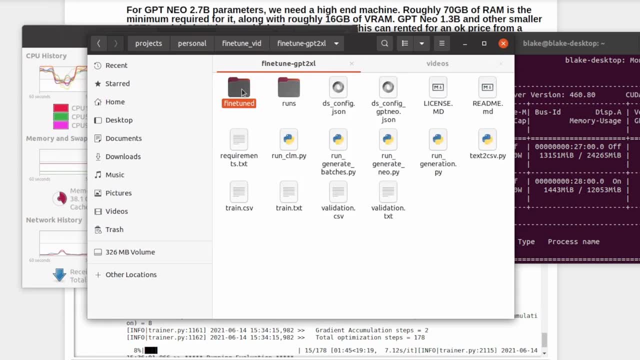 cheaper hardware that you can rent in the cloud in both of these cases whenever we're training a model the output of the model we're using the flies that we ran will be in the fine-tune folder 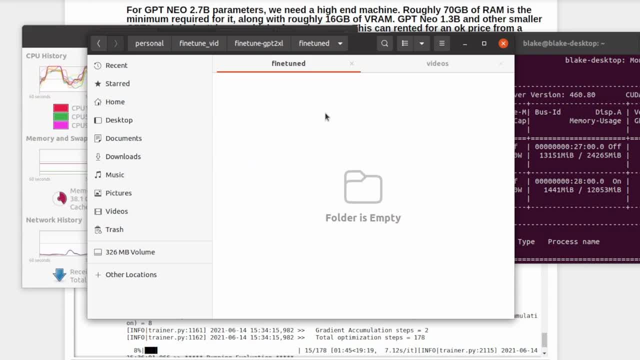 create default the flies that we use it will only save the last evaluation step so when it's done but 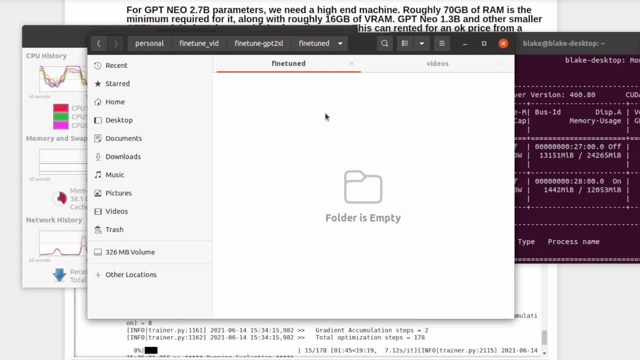 you can use flags that are described in the readme to have it save every epic or every two epics or Etc so this is where you will find the train model that you can use for later to end the video I want 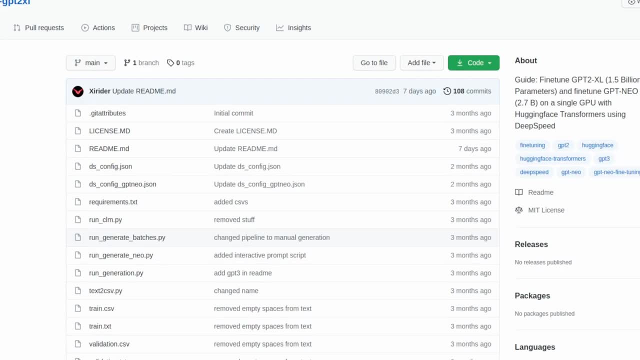 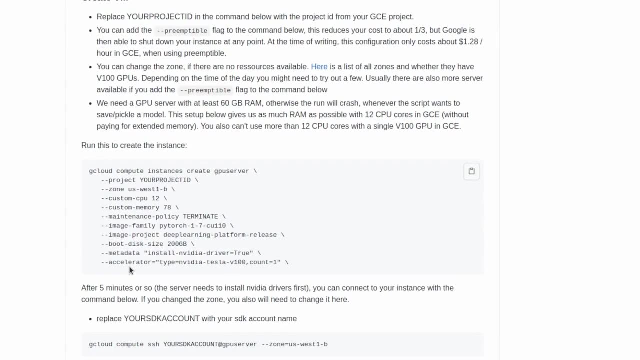 to briefly go over the GitHub page and the readme here we can see some of the steps to create a VM that I talked about if you don't have the hardware required and you can feel free to 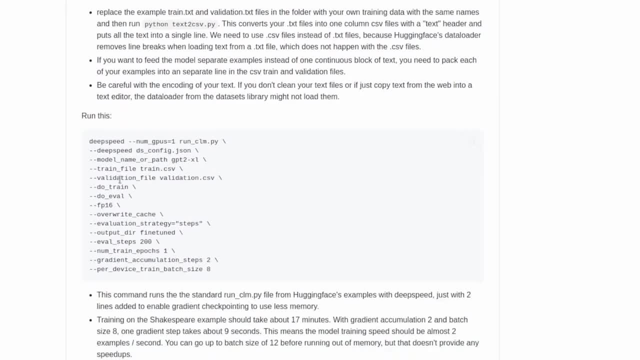 follow that or ask questions and I'll be happy to help here are some steps to fine-tune a GPT-2 2X 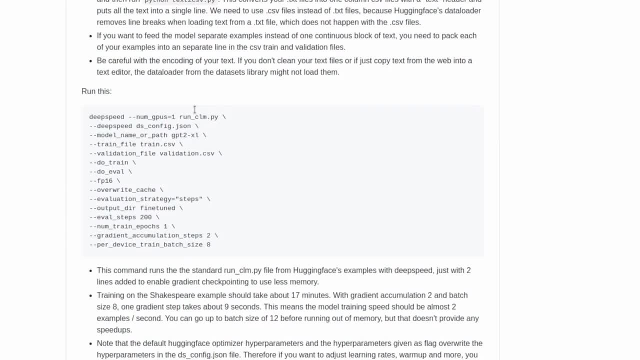 which is 1.5 billion parameters so if you're interested in that you also can do that it's very similar to what we did in fact the only difference would be instead of running the 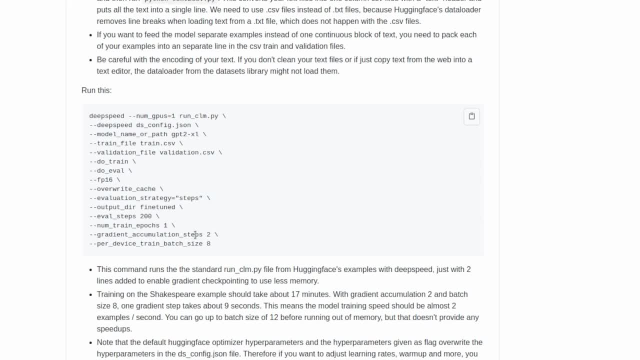 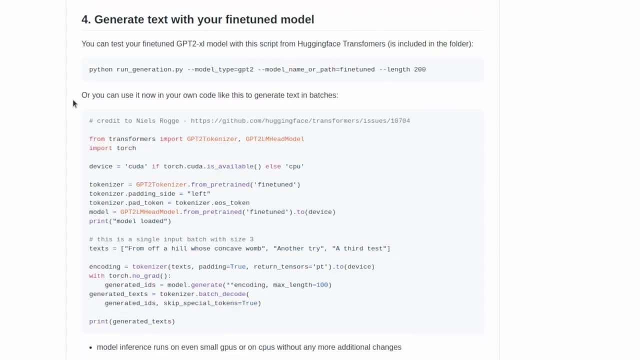 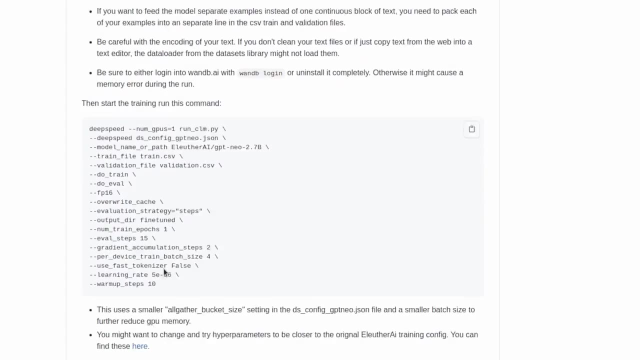 commands that we have in the Jupyter notebook you'll run these here we can see some steps on how to generate text with your fine-tune model this is for GPT-2X but it's similar for GPT-NEO here's the steps on how to train GPT-NEO and then here is the step to 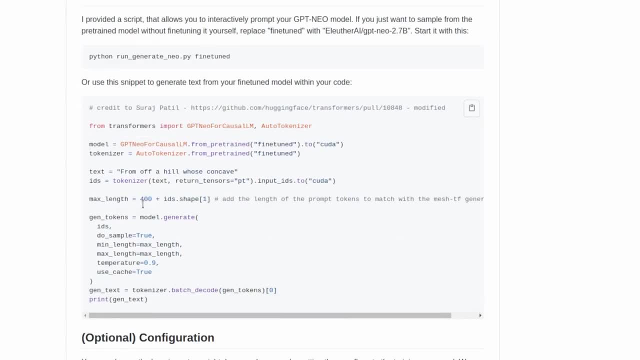 generate text with your fine-tune model I plan on making a another video on how to best generate text using your fine-tune model though this will work I have found that there are some few things 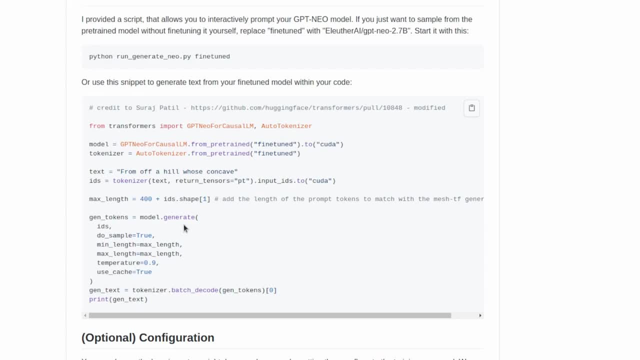 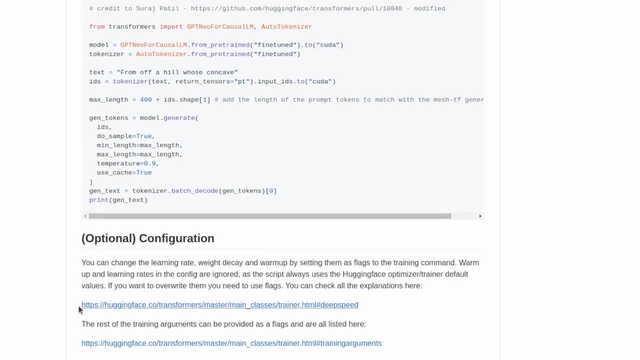 you can do just to make easier to play around with your fine-tuned model and lastly but still very importantly is the optional configurations I recommend looking at 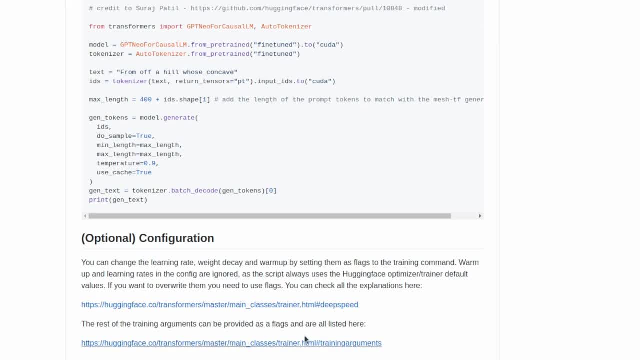 the training arguments that you can find the link on the bottom of this readme there are optional flags that you can append to this area here for training 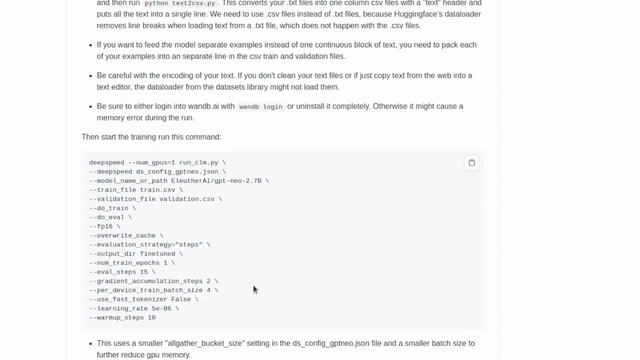 that will allow you to change how often a model is saved is it saved every 10 epics or 5x or whatever just things to make it easier to get the result you're looking for when training the model you're going to want to keep training 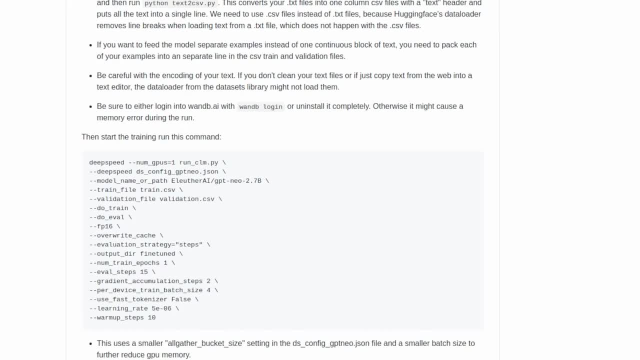 until your evaluation loss is the lowest that it can be at some point your evaluation loss will start increasing again so it's a good idea to stop once you notice that the evaluation loss has reached its minimum and it's starting to 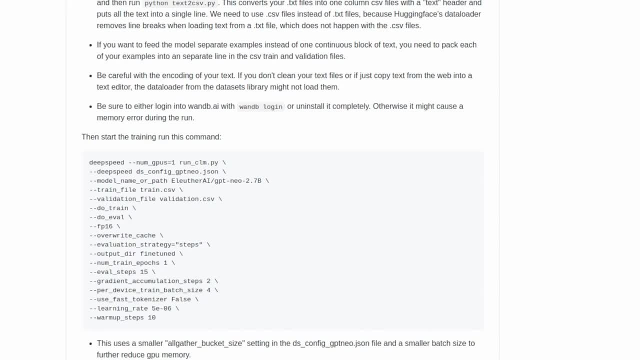 go up for me training on a custom data set not the one provided I found that it takes roughly four epics to get the best result so that's something you ought to play around with to find what works best for you so at 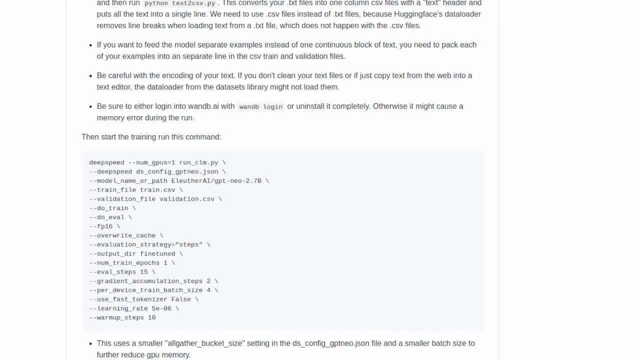 this point I'm going to end the video I hope that this video has helped you be able to fine-tune these very cool very large models for future videos I plan on 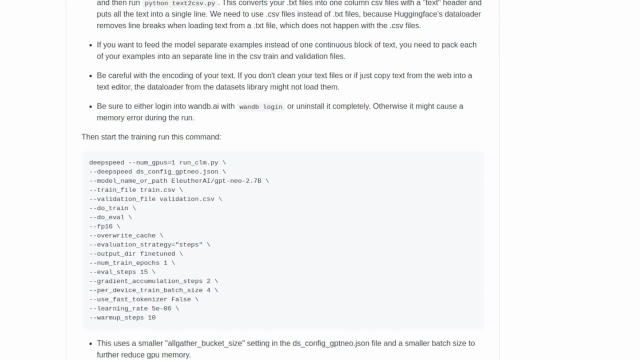 making a video on how to best use your fine-tuned model to get the outputs you want I also plan on making a video on fine-tuning a model on your own custom data set rather than just doing it on your own custom data set so that you can the provided data set so feel free to subscribe if that interests you so you 85% of adults have drank alcohol in their life. It's an extremely popular drug that decreases specific neuronal excitation in your brain, with biological byproducts that have a huge impact on your body. So if you're wanting to partake in a bevy short for beverage, is there an ideal time? for your physiology? Is it better to day drink or drink at night? When you drink a shot of vodka, 20% of the alcohol is absorbed by the stomach, 80% in the small intestine, where it goes into your bloodstream, then to your liver to be metabolized. Ethanol gets into cells by passive 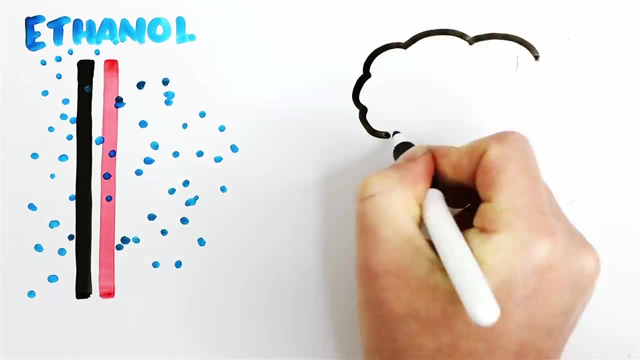 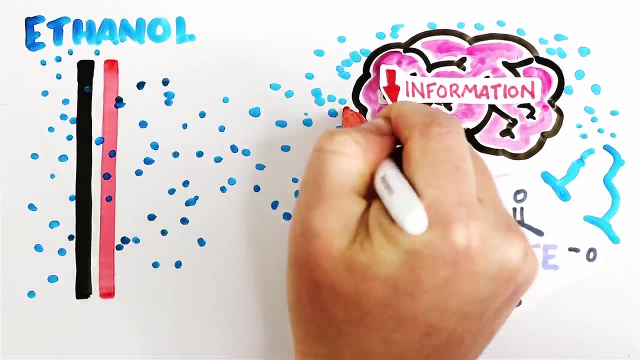 diffusion. so the more you drink, the faster you get drunk. And when alcohol accumulates and finally gets to your brain, it suppresses the excitatory neurotransmitter glutamate, which causes information transfer in the brain to become slower, with only the largest signals making it through.